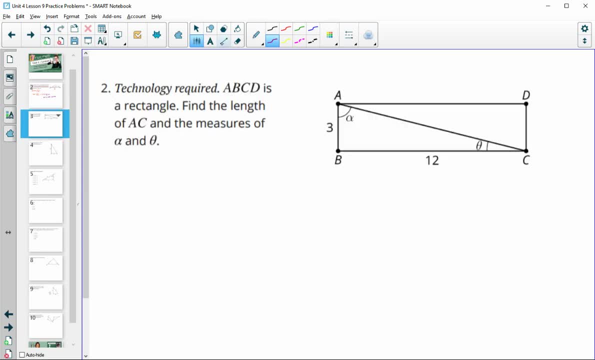 Number two: find the length of side AC and then find the missing angles. So AC is the hypotenuse here of a right triangle and because it says that it's a rectangle, so rectangle means we know that these angles are 90.. 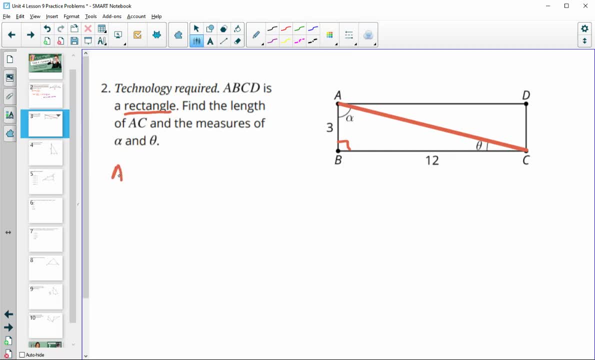 So we're going to be able to do the Pythagorean theorem. So AC squared is equal to 3 squared plus 12.. So 12 squared 3 squared is 9.. 12 squared is 144.. So AC squared is going to equal 153, and then we will square root that. 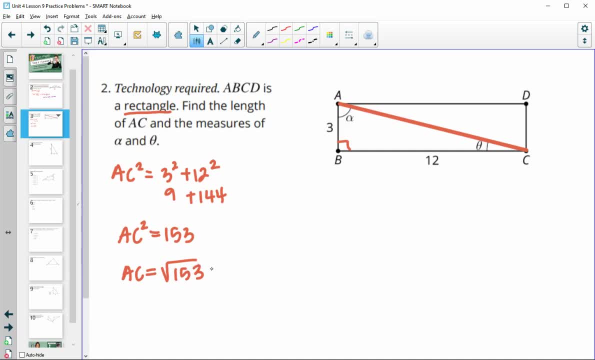 So you can either leave it as square root of 153, or you can do a decimal of 12.4.. Then we need to find the measure of these angles. So I'm going to find theta first, So I'm going to be looking for this one. 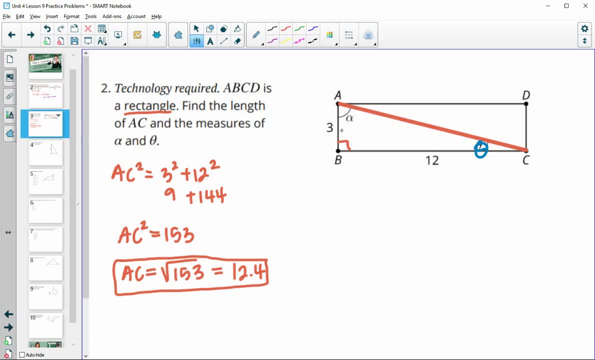 So I'm going to label the sides based on this angle. So across from the theta is the 3, so this is my opposite side. The 12 is next to it, so the 12 is the adjacent side. So I'll be setting up an arctan function, since I have opposite and adjacent and I'm looking for the angle. 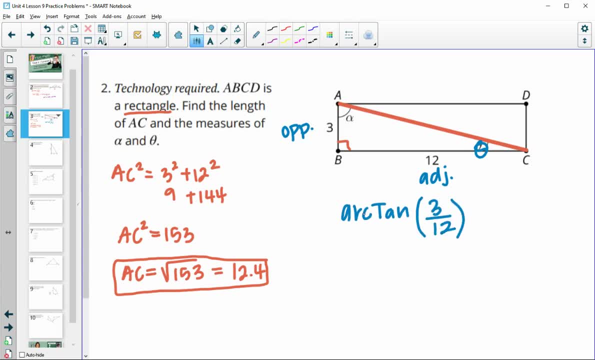 So opposite is 3, adjacent is 3.. The tan is 12.. Again, this is also the same thing as tan negative 1 in your calculator. So type in the arctan or tan negative 1 of 3 divided by 4, and you get 14 degrees. 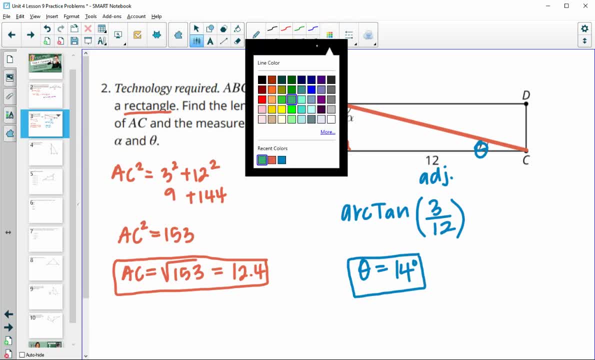 Then, when you go to find alpha, you can set up an arctan of 12 over 3. You flip these around, since this would be the opposite. So this would be the opposite of the alpha and this would be the adjacent. 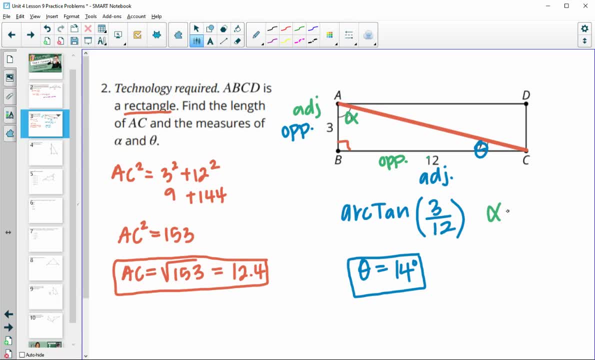 So you can do another trig function. You can also remember that alpha would be equal to 90 minus theta, since these two are going to total 90, and theta is 14.. So 90 minus 14 is 76 degrees for alpha. 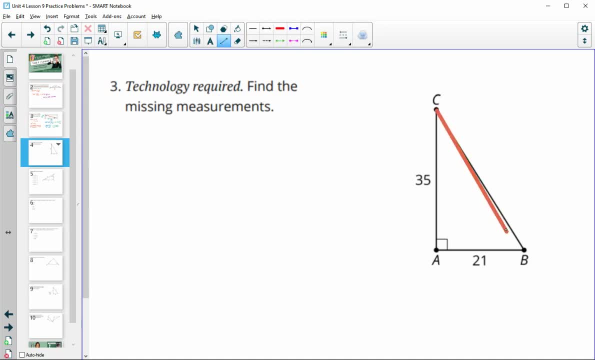 Find the missing measurements in Number 3. So we're going to need to find this hypotenuse again and then find angles B and C. So a very similar problem to number 2.. So finding the hypotenuse here, 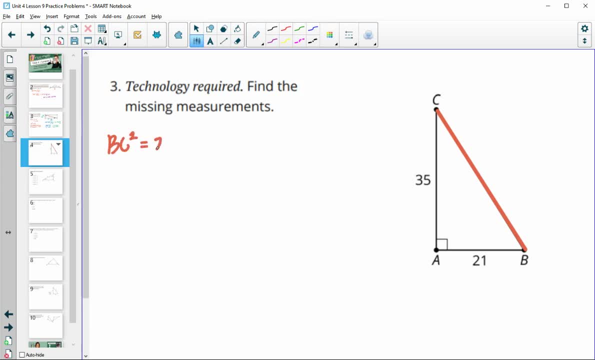 So BC squared is equal to 35 squared plus 12 squared. 35 squared is 1,225.. Oh, not 12 squared, Sorry. 21 squared And 21 squared is 441.. So add those together and you get 1,666.. 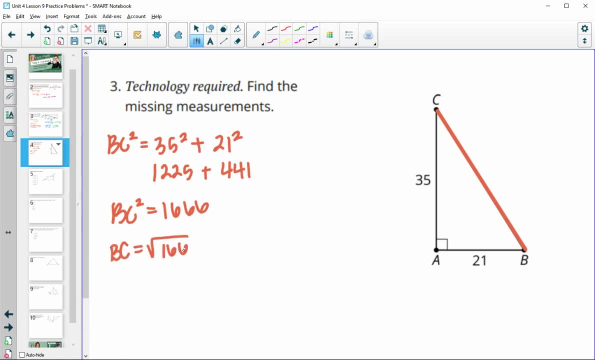 So then we will square root that and we get 40.8.. So then we need to find the different angles here. So I'm just going to find the angles here. So I'm just going to find angle B first. 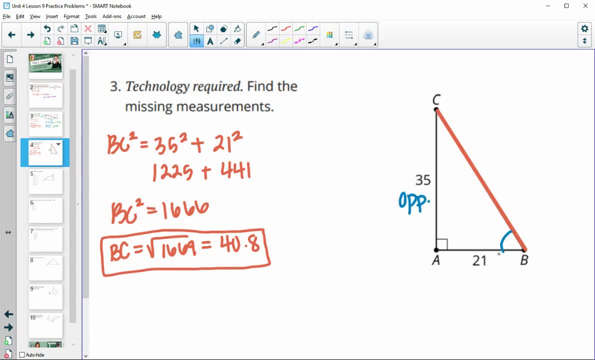 So across from B is 35. So that's our opposite side. Next to B is the 21. So this is our adjacent side. So this is going to be an arc tan to find the angle, or a tan negative 1.. 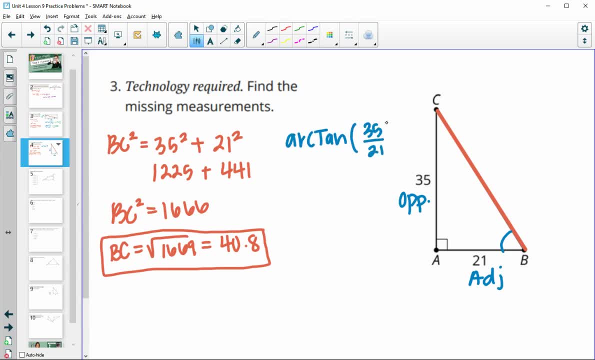 So opposite is 35. Adjacent is 21. So angle B is going to be equal to 59 degrees. And then to find angle C, we'll just subtract 59 from 90. So we'll do 90 minus 59, and that will give us angle C which is 31 degrees. 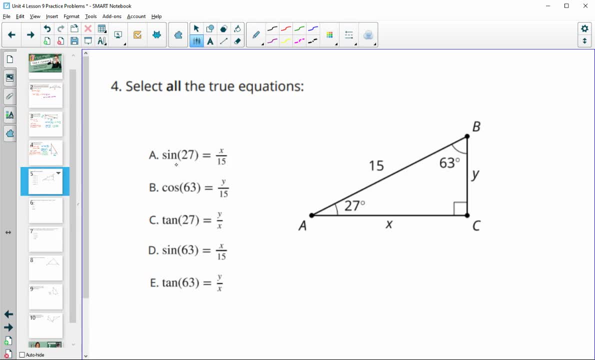 Number four: select all of the true equations. So A says the sine Sine of 27.. And remember, sine is the opposite side, Y over the hypotenuse 15.. So this one is not true because this one did the adjacent over the hypotenuse. 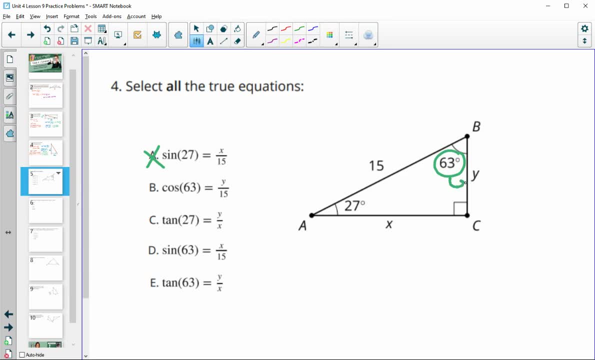 Cosine of 63.. So cosine is the adjacent side, which would be Y, in this case over the hypotenuse, which would be 15.. So Y over 15 is good. C is the tangent of 27.. 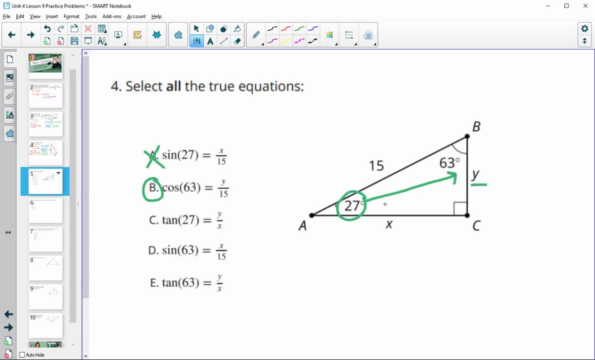 So tangent is the opposite side, which is Y, over the adjacent side, which is X. So tan 27 equals Y over X, is a true statement. D is the sine of 63. So here's 63. Opposite side would be X. 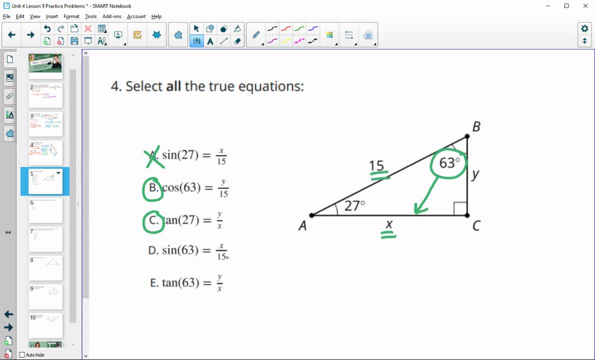 So sine is opposite over hypotenuse, which would be X over 15.. So this one is good. And then tan 63 would be the opposite X over the adjacent Y. So they have this one flipped around. So this one is false. 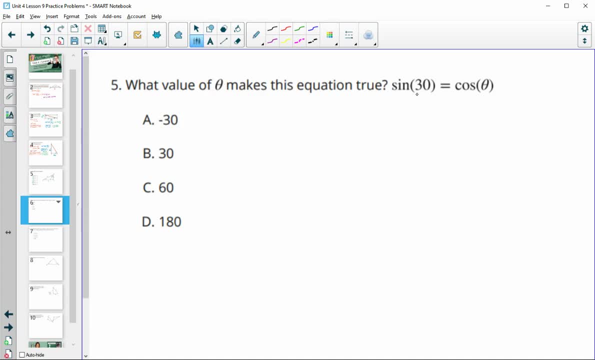 Number five: what value of theta would make this equation true? So remember sine and cosine. if these numbers add to 90, then they're equal to each other because they'd be opposite kind of angles in a right triangle. So we know that theta would equal 90 minus 30. 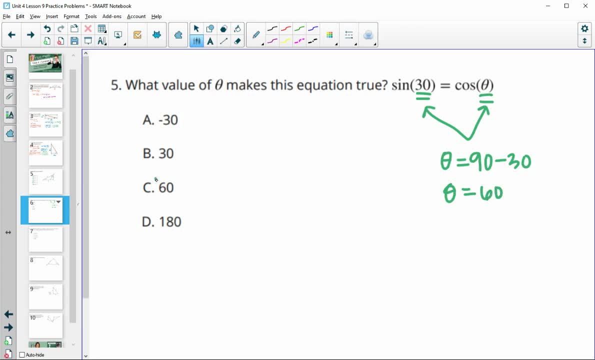 So theta is going to be 60.. And then these would be the same. Then the sine and the cosine would equal each other. Number six: a rope with a length of 3.5.. 5 meters is tied to a stake in the ground. 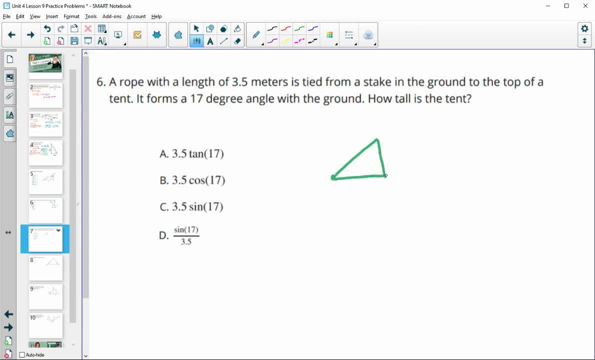 And at a 17 degree angle. So we know this angle here is 17.. The hypotenuse is 35. And we're looking for an expression for how tall this tent is, And so when we have this angle, the opposite side of that angle is this height. 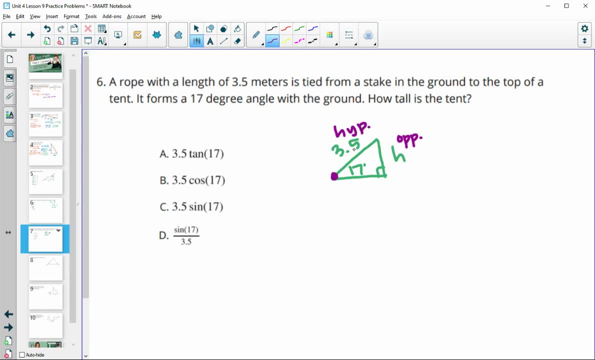 And the 3.5 is the hypotenuse, Since it's a cross, So we can set up a sine function. So sine of 17 would equal the opposite over the hypotenuse. And then if we cross, multiplied here or multiplied that 3.5 up. 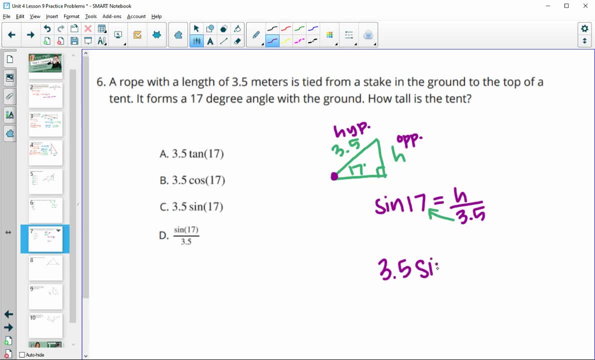 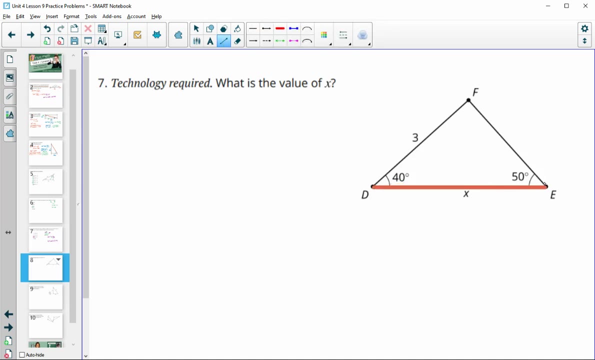 we would get 3.5 times the sine of 17 would equal H, And that is option C, Number seven. What is the value of X? There's going to be multiple different equations that you can set up here, depending on which angle you would like to use. 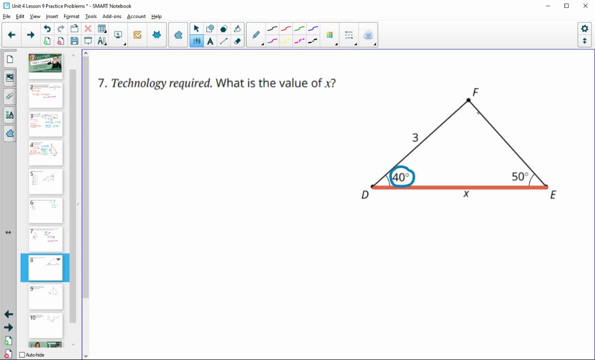 I'm going to use the 40 degree angle. So then we see this is 40 and 50, which total 90. So we know that this angle is a 90 degree angle. So we'll be able to use trig. 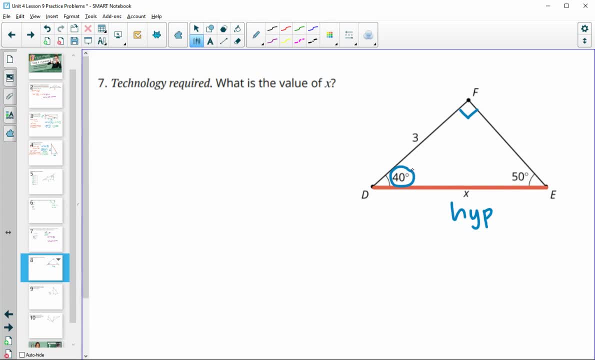 The X is the hypotenuse. Since I chose this 40 degree angle, the 3 would be the adjacent. So I'm going to be setting up a cosine function. So cosine of 40 equals the adjacent side 3 over the hypotenuse X. 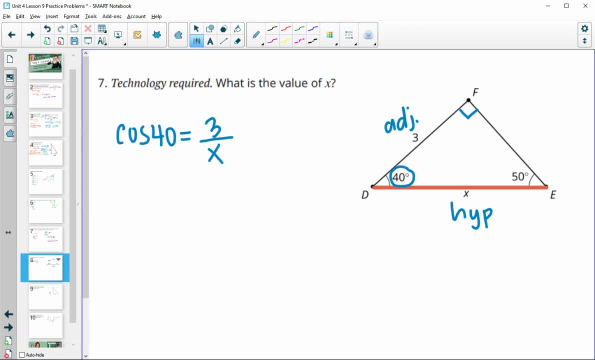 And so then cosine of 40, we'll type into our calculator and we get 0.7660 equals 3 over X. We'll multiply this X up, So we get 0.7760.. X equals 3.. 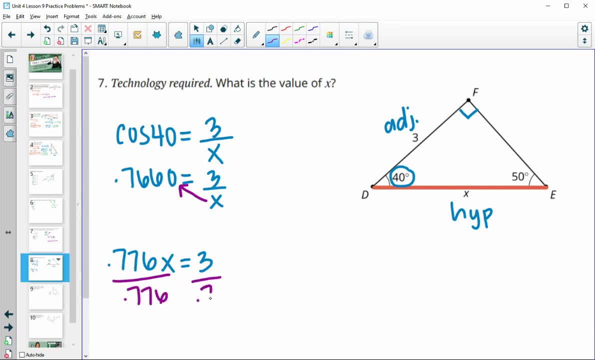 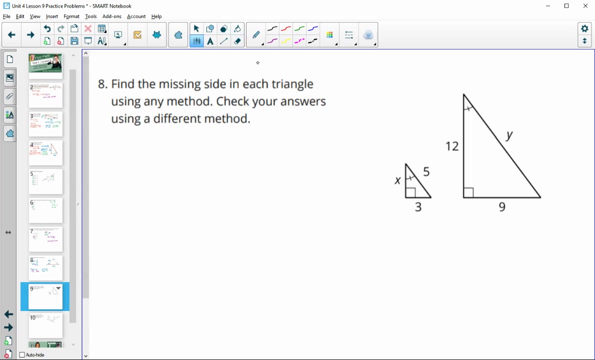 Divide by 0.776.. And we get that X equals 3.9.. Number eight: Find the missing side in each triangle using any method that you would like. So we do. We do see that we have right triangles here and we have two out of three missing sides. 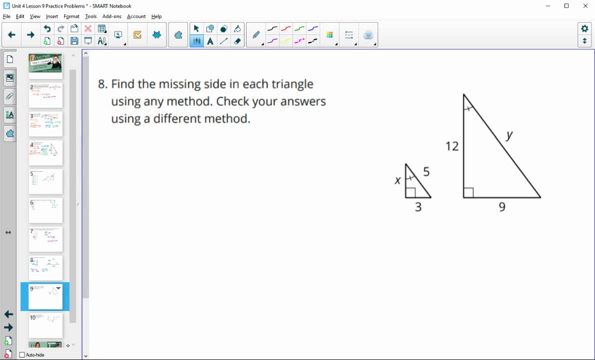 or two out of the three sides, So you could certainly use Pythagorean theorem. We also see that we have a 90 degree angle and another congruent angle, So we know that these triangles are similar. So Pythagorean theorem would be fine, or similar, like or using scale factors. 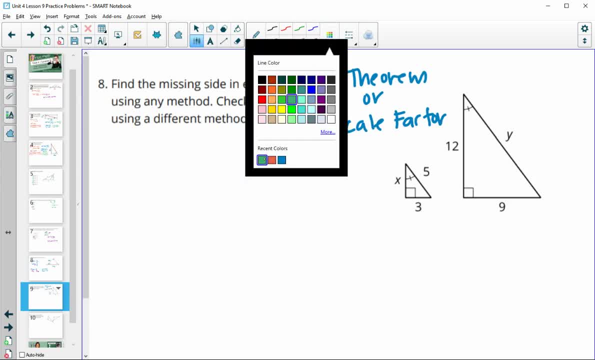 So I am just going to use scale factors. So I see that this side is similar to this side. So if I'm going from the small triangle to the big triangle, then the scale factor is going to be multiplying by 3.. 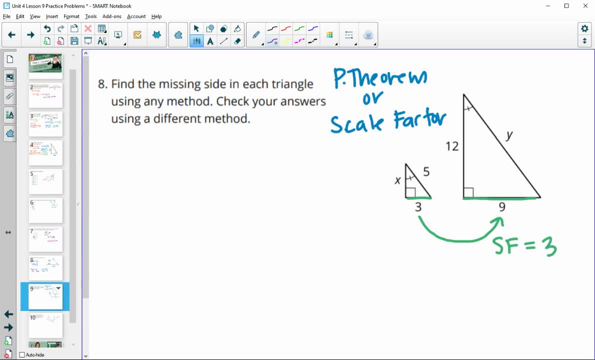 And if I'm going the other way, then it would be dividing by 3.. So if I'm going from this 5 to this Y, okay, the Y is larger, So it's going to be 5.. So if I'm going from this 5 to this Y, okay, the Y is larger. 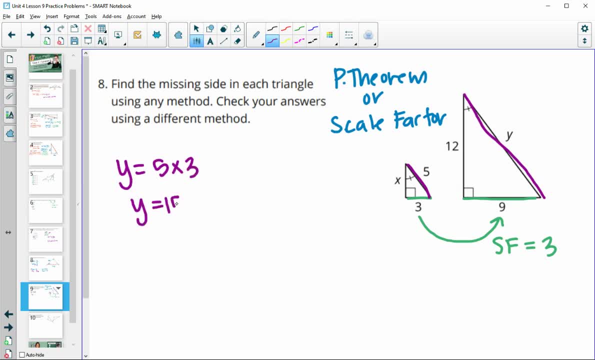 So if I'm going from this 5 to this Y, okay, the Y is larger times the scale factor of 3. So the Y is equal to 15.. And then when I'm going from 12 to X, so that one's getting smaller,